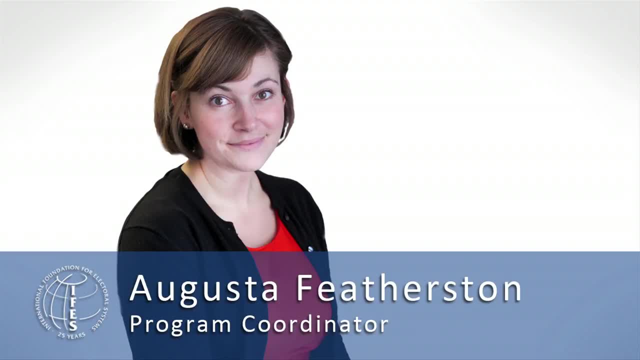 to address that problem and they might know how to mobilize resources within the community. They might know how to organize others who are sympathetic to the same cause. You know those things. You know those are rules of engagement in our society that no one is born with. They're nurtured. 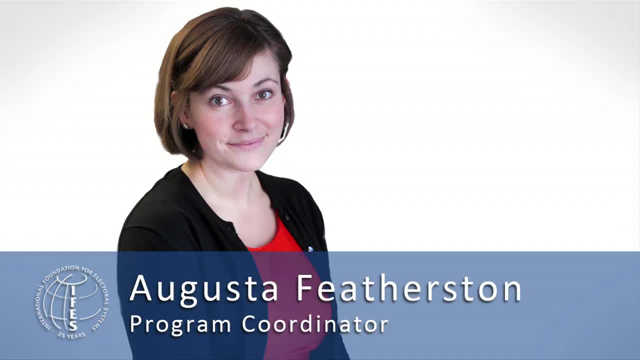 over time. What are some of the challenges to implementing these programs and how do you overcome them? I think one of the challenges that practitioners face quite frequently comes from, you know, getting an appropriate level of buy-in from families. Oftentimes, youth programs are specifically. 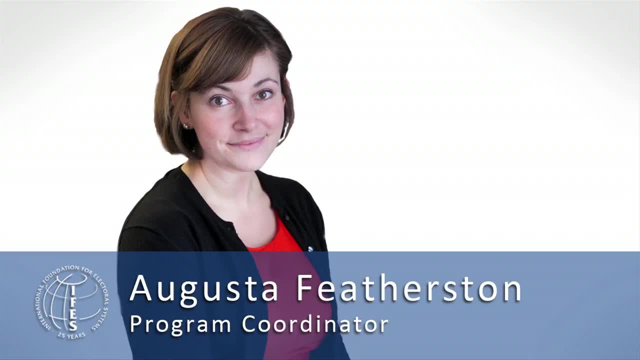 targeted towards students who, for the most part, are marginalized. You can have a great concept for an innovative youth program, but if the content and activities are something that parents or guardians are not on board with, you'll never be able to have the young people. 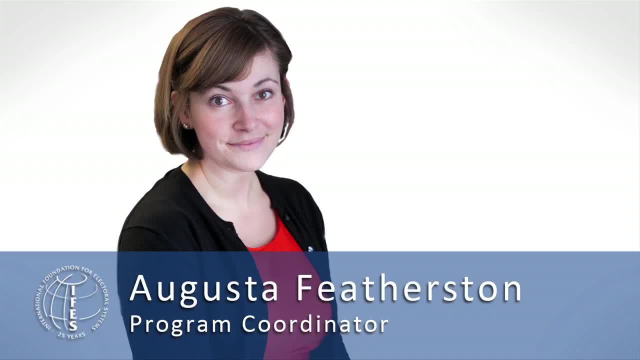 participate for any meaningful amount of time. You know so one way to address this challenge is by making sure that parents, families, guardians, whomever- are included in the planning process, or at least they're given every opportunity to know about the program and what it entails. Another challenge is just having 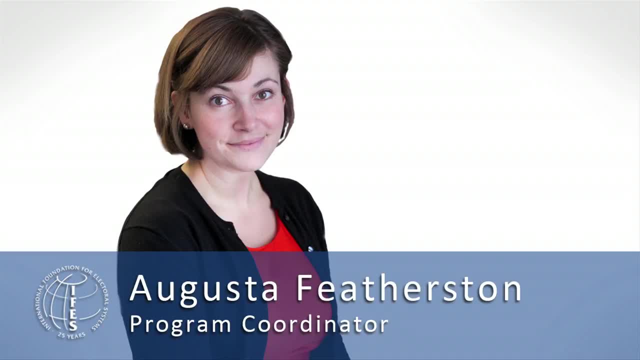 enough time with youth participants. In my experience, young people sometimes start attending a program and then later simply stop showing up. So sometimes you'll know it's because the student has joined a different activity or maybe the family moved away. One way that I've found to mitigate this particular challenge is by 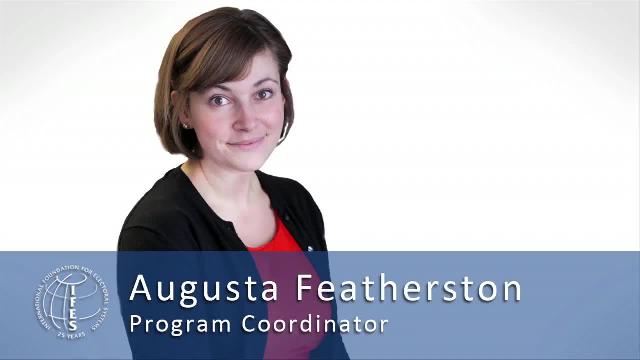 making, just making the most of the time that you do have with the students. So there's no wasted time in a program. Every, every moment can be a teachable moment. What are some of the programs that IFAS has implemented? We've implemented several different types of programming around the world. One of the flagship youth programs that IFAS 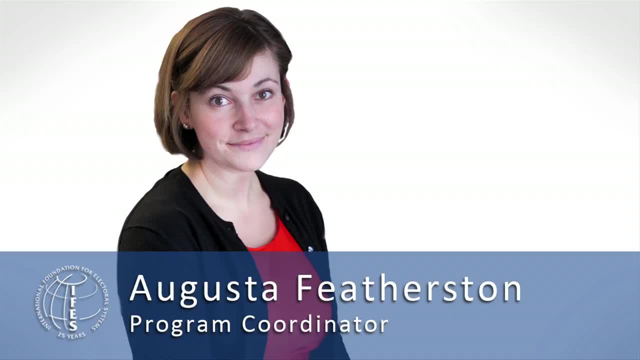 implements are democracy camps in Kyrgyzstan. These are camps geared towards high school-age students throughout the country. They come together for about ten days and they work their way through a curriculum based around simulations, small group exercises, theater. It's been running for quite a long time.